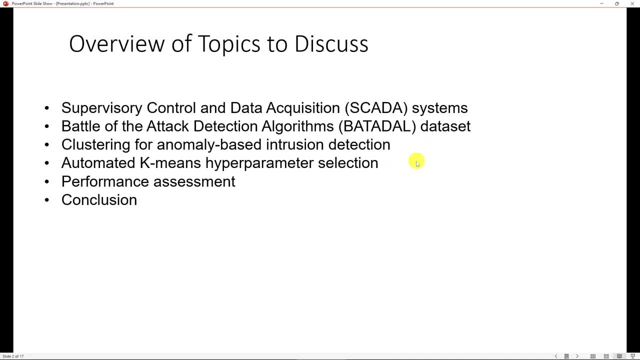 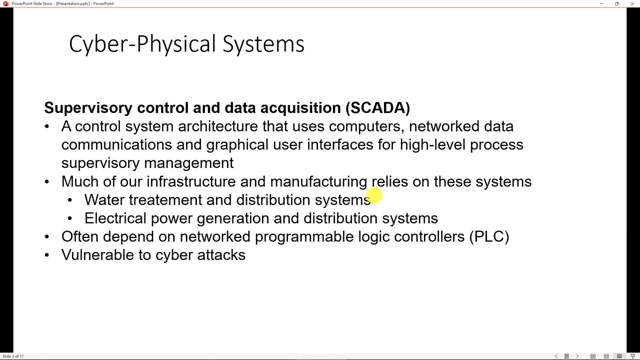 And then I'll talk about the performance assessment metrics and the actual results. Okay, so these cyber-physical systems that we're going to talk about today, We're going to be looking at here, use supervisory control in data acquisition systems. So it's a collection of computers, network data, communication, graphical user interfaces, etc. 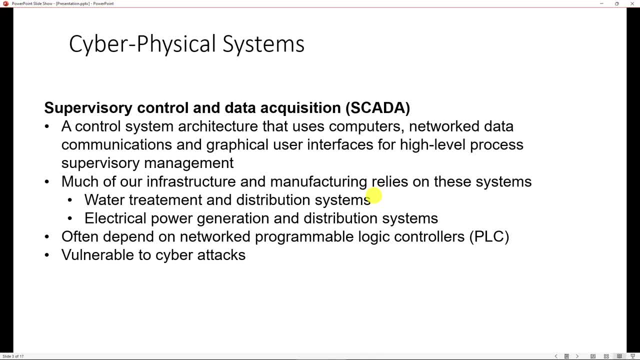 For supervisoring various critical infrastructure systems. So water treatment systems, water distribution systems, electrical power generation and distribution, A lot of manufacturing and just large-scale infrastructure Use these cyber-physical systems that rely on these SCADA systems. Unfortunately, as these become networked with these programmable logic controllers, they become more susceptible to cyber-attacks. 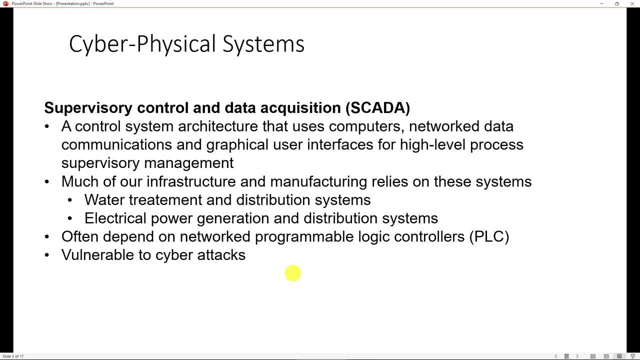 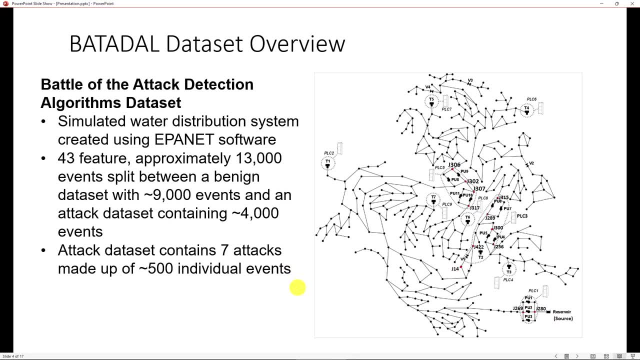 So we're going to be looking at ways to detect those. A little bit about the dataset. we're going to be looking at The battle of the attack detection algorithms, The algorithms dataset. So this is simulated using Epanet software, which is just a water distribution system software. 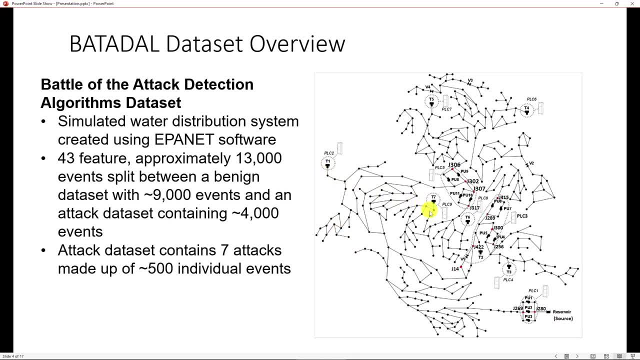 You can see the network map. We've got a collection of water tanks, various PLCs connected to those tanks, as well as valves, junctures or junctions, And we collect all kinds of different data from these: flow rates, Their status, whether they're on or off, etc. 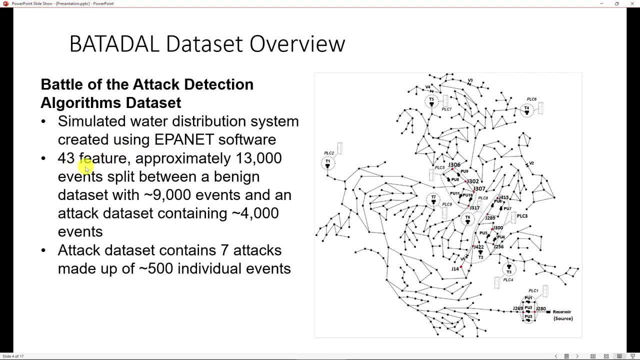 There are 43 features in this dataset- approximately 13,000, split into two separate datasets: One is 9,000 events, or 9,000 rows of benign operating data- normal operating data, And the other one is 4,000 events, some of which correspond to attacks. 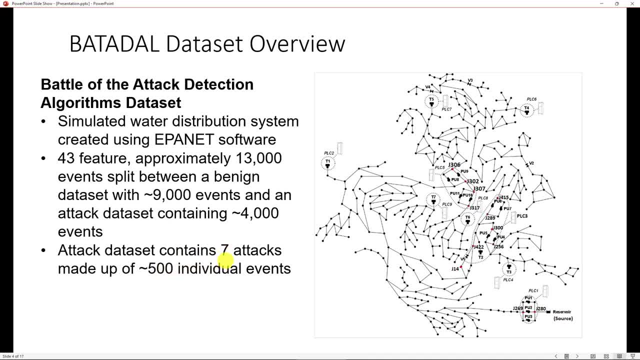 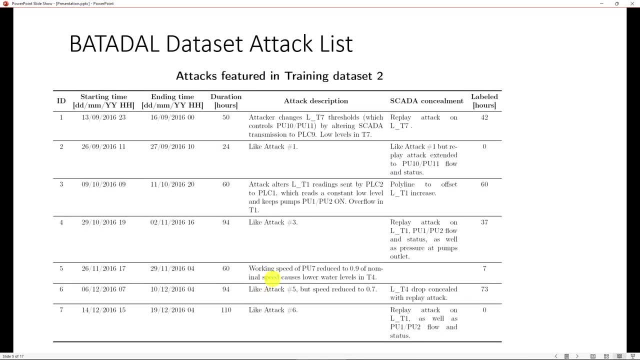 Specifically 500, about 500 events spread out over seven different attacks. We also have a list of those attacks, So we've got the attack duration for each of these. So this will be 50 events, one after the other, 24 events, 60 events, etc. 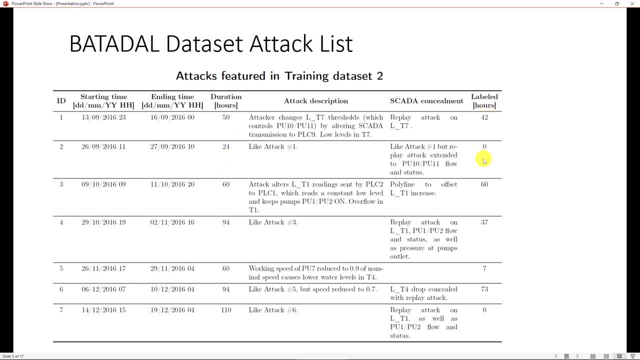 These were not initially labeled in the dataset. However, for the purposes of assessing these, we did go in and include these labels During the training. we don't use any labels at all, but we do use them for assessment. So you can disregard this column. 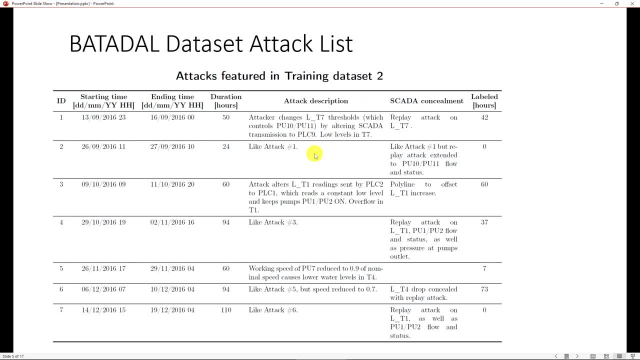 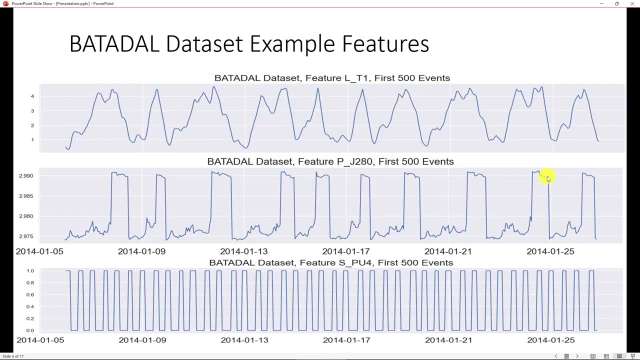 And then we've just got some descriptions of what happens during the attack. A lot of them are altering the transmission of information to the SCADA system just to hide the fact that this is going on. An example, just a selection of features from this dataset. 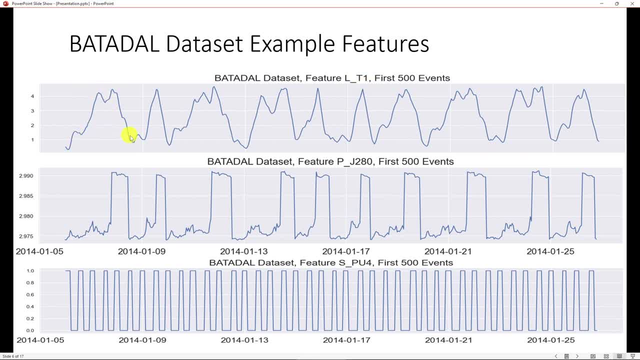 Here we have the level of tank 1. This is pretty ordinary looking continuous data stream. Similarly, we've got the junction 280 here. We've got the flow rate here or the pressure in that. You see, it's slightly seasonal, just a different pattern here. 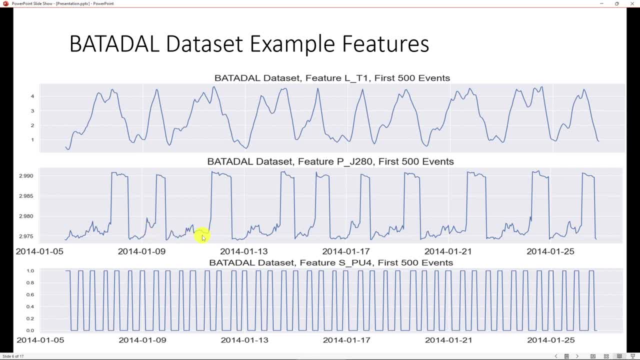 We've got altering from periods of low pressure to high pressure, with very little in between, And then, finally, we have purely binary data. This is the status of one of the pumps that alternates between 1 for the pump being on and 0 for the pump being off. 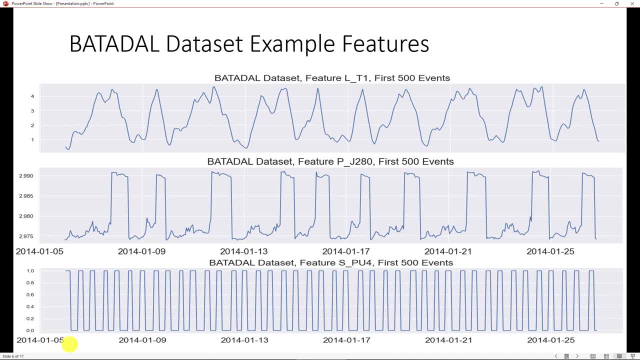 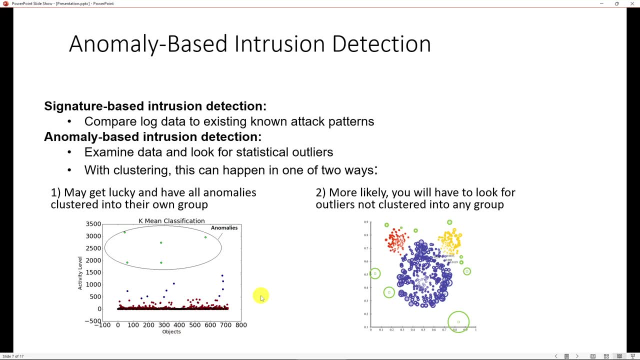 So kind of the different types of data we've got going on here. Okay, just a quick introduction to the anomaly-based intrusion detection. Most systems, like your standard virus scanner on your computer, uses a signature-based intrusion detection method where your log data is compared to the existing attack patterns of known attacks. 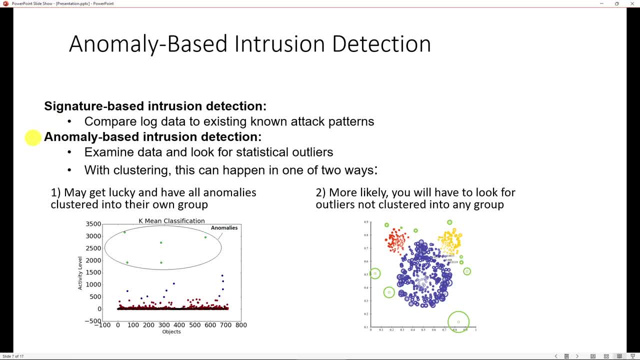 So something that has been seen before: Anomaly-based intrusion. on the other hand, we want to look at data and kind of establish what normal data looks like and look for statistical outliers of that data. So, when performed using clustering, this can happen in a couple of ways. 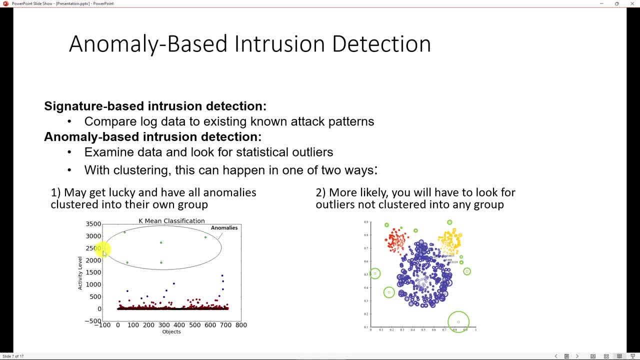 Either you're lucky and your classifier will group all of the anomalies in their own cluster. So here we've got a green cluster with all the anomalies, a blue cluster, a red cluster, etc. That is not likely to be the case. 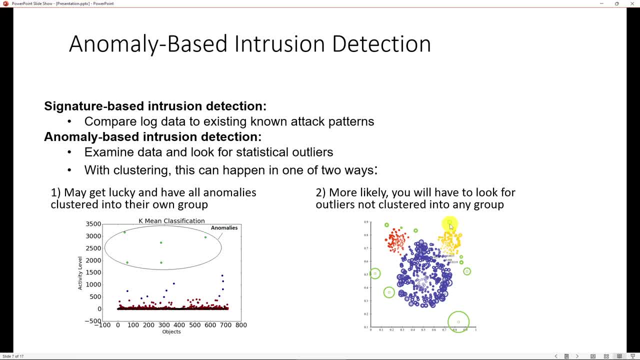 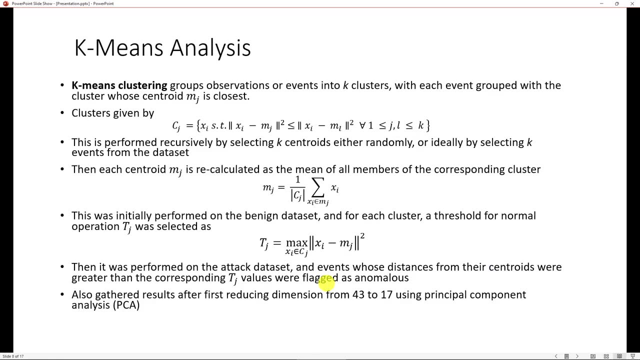 Most often you have your clusters and then your anomalies are outliers of those clusters. So that is the case with this data. So once we've established our clusters, we just look for things on the fringes of those. So an overview of k-means clustering itself. 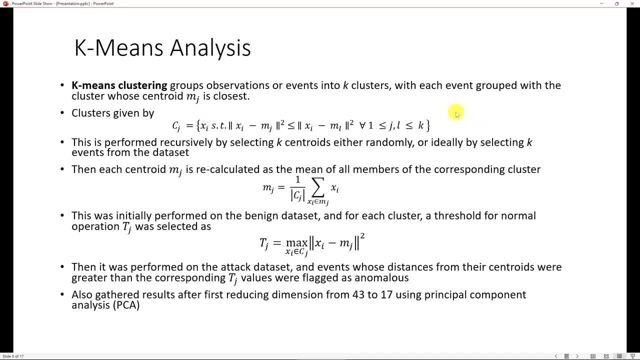 What we're doing. each this is a recursive model or clustering method, in which a collection of k clusters are chosen. Typically, these, the centers of the clusters, are what's chosen, either randomly or by selecting k elements from within the data set. 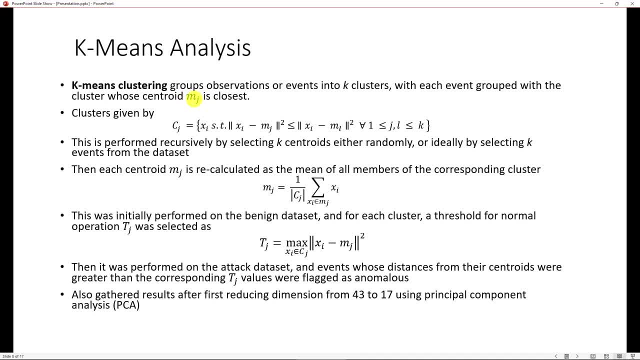 and making those your cluster centers And then just finding the points that kind of minimize. excuse me, you're looking for the for each data, point x, i. you're looking for the centroid that is closest to it. So we find the distance between each of these centers. 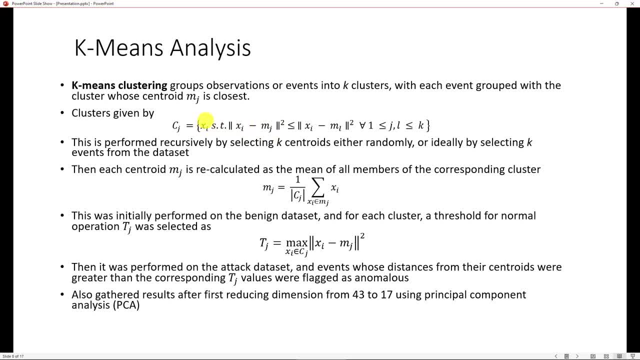 and just select the smallest one. The collection of all points corresponding to that center make up that cluster. Once that is performed initially, this is repeated just by finding the average or the mean of all the points within a given cluster to find a new centroid. 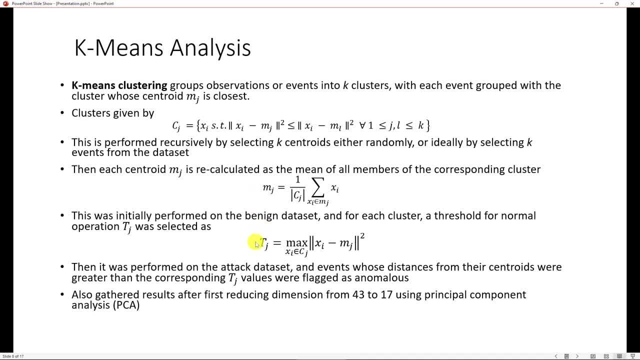 And this process is repeated. Finally, in order to find these thresholds, like we talked about in the last slide, we're looking for outliers within our clusters. All we did is we performed this k-means clustering on the benign data set and found the max distance. 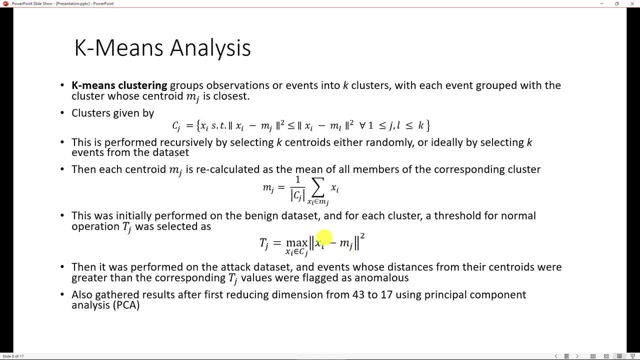 For every centroid. we looked at each point within that centroid and just found the max distance here And that was our threshold. Then we performed the same thing on the attack data set and just looked for any events that were outside of this threshold. 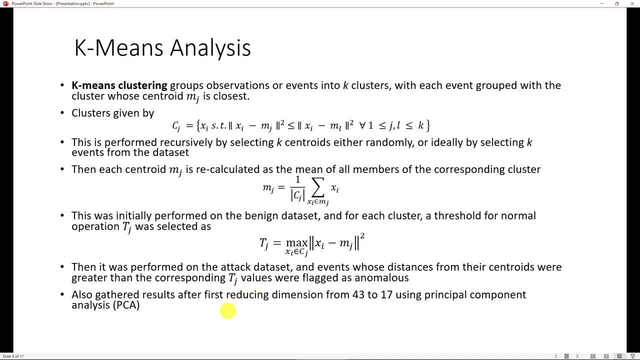 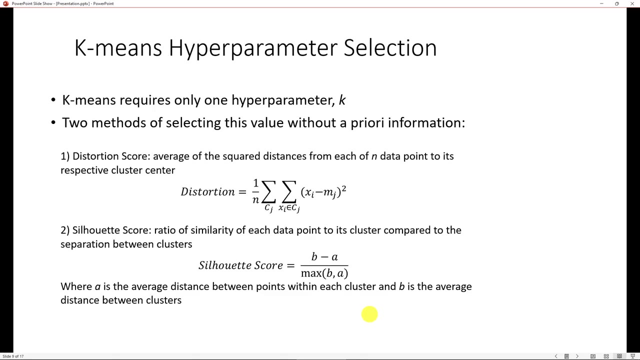 for each centroid. Finally, we also tried this. we performed PCA, first to reduce the dimension, and we ended up, I believe, using 17 components down from 43, to see how that affected the results. Okay, so, in this type of model, 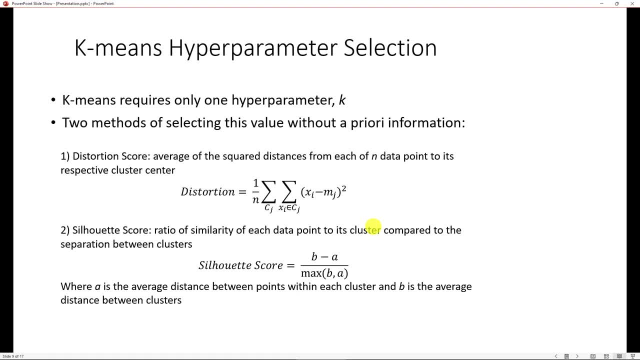 ideally we want to select the hyperparameters without any information about what's going on or whether or not there's an attack happening. We don't want to analyze the results and then kind of work backwards and see: well, what's the best result? 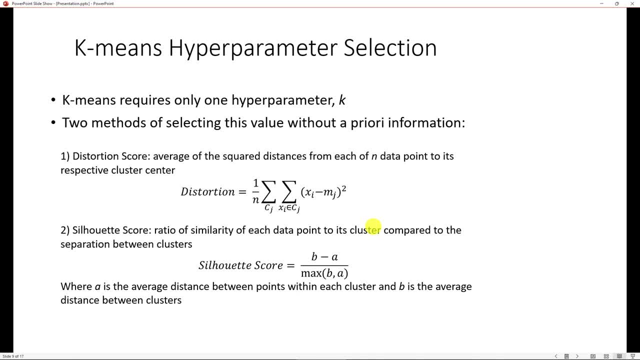 We do do that. We do a grid search where we check all possible parameters for either PCA or k-means or both together, just to compare our results. But we want a way of doing this ahead of time. So the two methods of doing this: 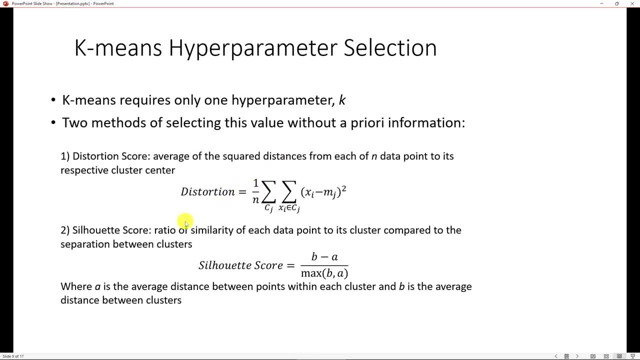 are the distortion score and the silhouette score. The distortion score is the average of the squared distances from each of the end data points to its respective cluster center. This one is relatively straightforward to calculate. And then, finally, we have the silhouette score, which is the ratio of the similarity. 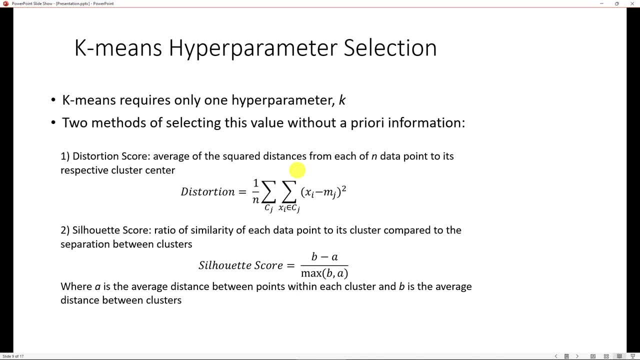 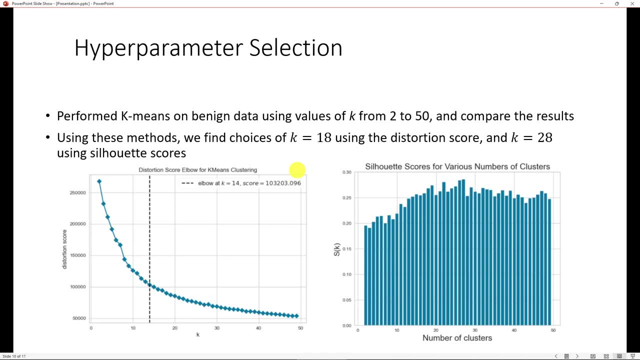 of data points to their cluster, compared to the separation between the clusters. So, looking at these results, we've got this distortion score and this has another name- It's escaping me right now- The sum of squares error. So we're looking at this distortion score. 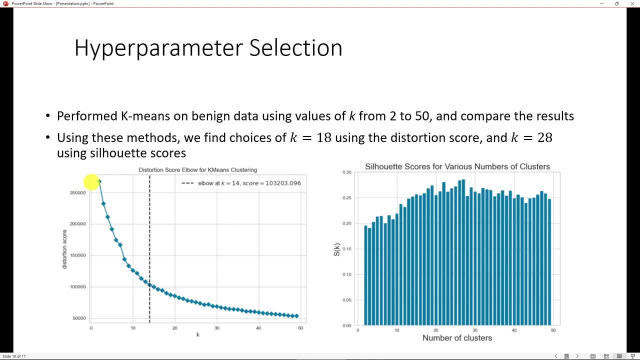 for each, each element of the data set for its cluster, and averaging these together and looking for not necessarily the lowest value, but the point where this curvature, where this curve changes drastically. They call this the ELBO method. We just select the point of maximum curvature. 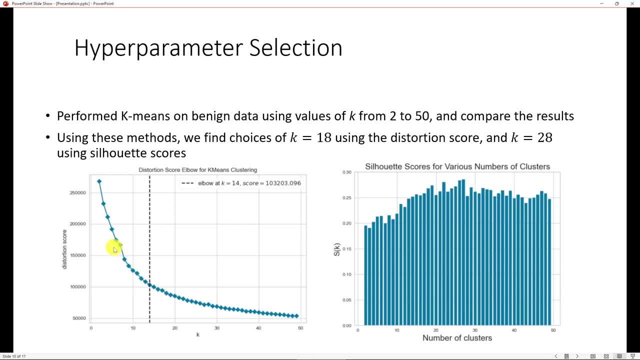 because here it's not really clear where the ELBO is happening, where this occurs, but you can calculate where this curvature kind of tapers off. So that happens when we have k equals 18 clusters. So we select 14 clusters based on this method. 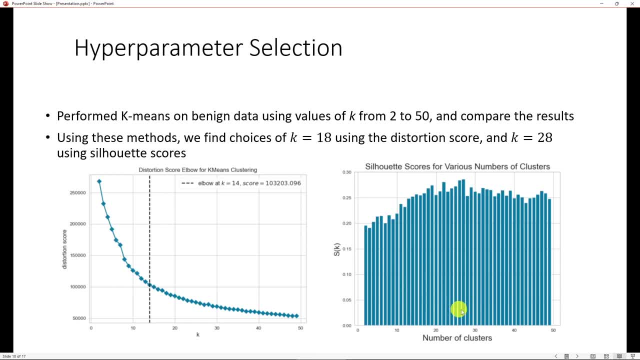 Using the silhouette score. we're just looking for the number of clusters. that gives us the highest silhouette score, which happens right here at 28 clusters, Although you see that there's not a whole lot of variation here. So in reality, a lot of these different numbers would work. 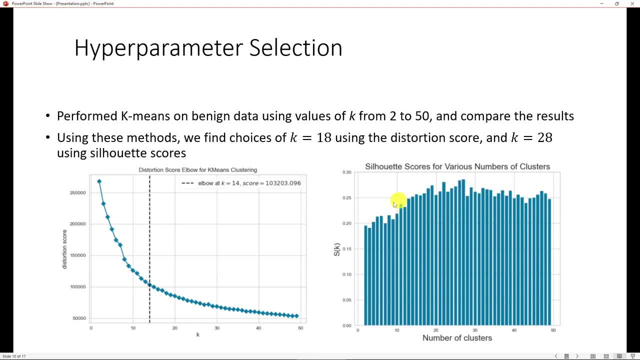 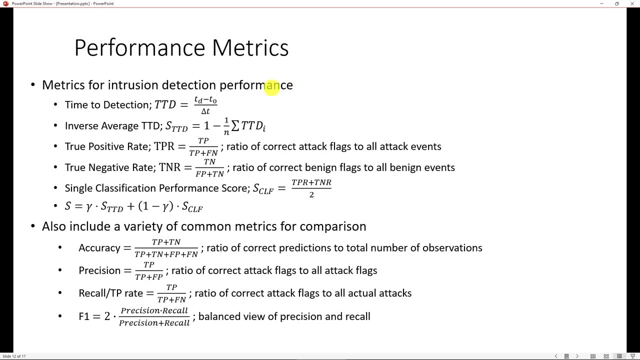 There are a few that are less ideal, especially these earlier ones, if you have fewer number of clusters, But in general these work similarly well. Okay, performance metrics: We use some ones that are less standard when it comes to machine learning in general. 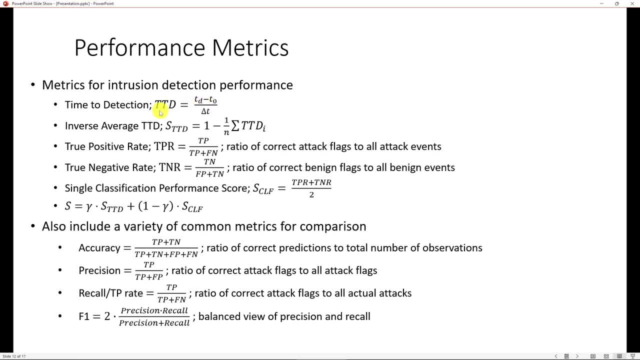 but are very important for intrusion detection. Those are time to detection, which is just the point in which an attack is first detected, And from that we subtract the start of the attack and then divide by the total length of the attack to get this time to detection. 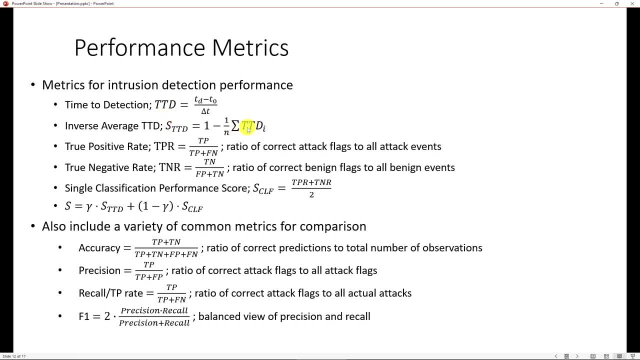 We also look at the inverse average of this. So we average all of these times the detections for our seven attacks. We take the average here just because the way this works- time detection, a low number, would be better, But taking this kind of inverse, 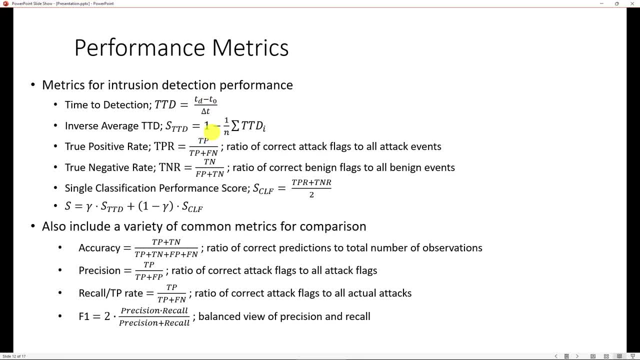 we can say: this is more intuitive, So now a higher number is better, And also that allows us to then use that later to create a single classification, a single score here, where again larger is better. So our STDTD is our kind of inverse. 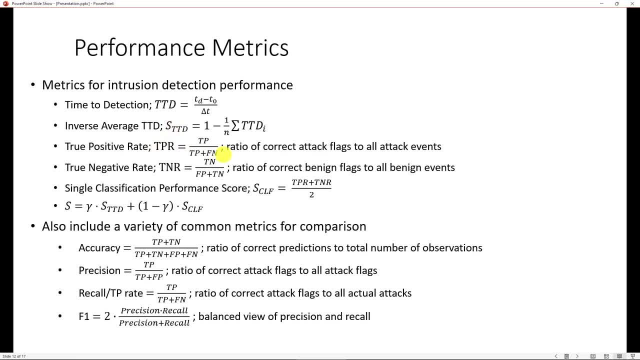 We also look at the true positive rate, which is the ratio of correct attack flags to all attack events, The true negative rate, the ratio of correct benign flags to all benign events. To get the single classification performance score, we average those together. 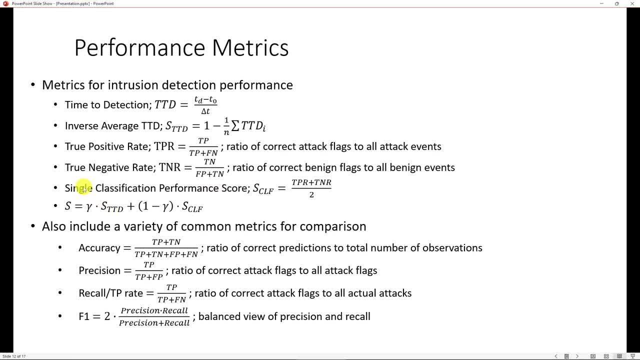 And then we weight these two things together. So this is like the classification performance and this is the time to detection performance, And then we weight those just depending on what's more important. In this case, we gave them both the 50% weight. 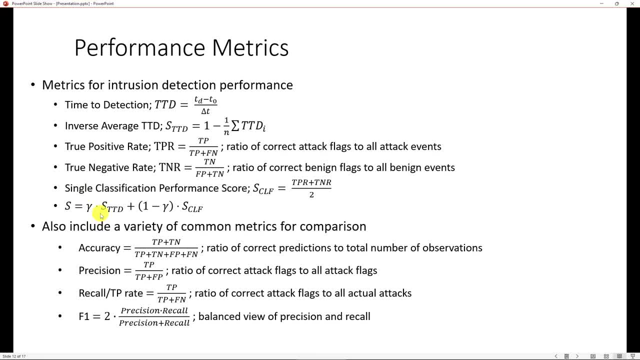 So gamma here is 0.5.. And additionally, there are all of these things called the standard metrics for machine learning comparison that are useful but not as important, because they don't include any method for time detection, which is one of the most crucial parts. 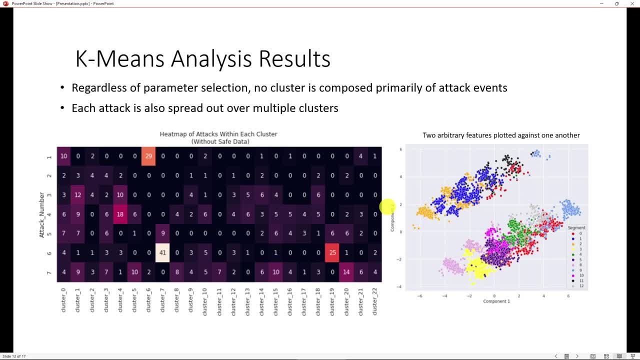 of this type of system. So looking at the analysis again, this just kind of repeats what we saw or what I claimed before. The attacks are spread out between all the different clusters, So like for example, in cluster seven, you see there's four attack events. 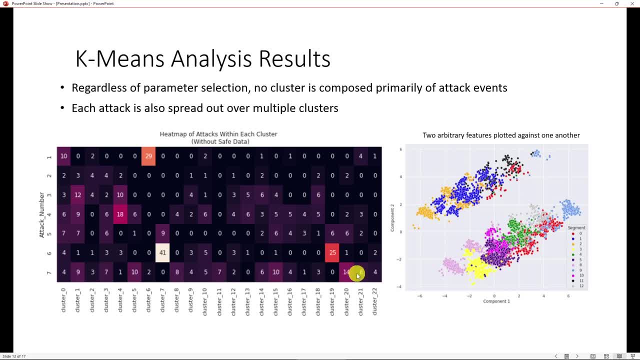 in cluster zero, nine in cluster one, etc. So each attack is spread out over multiple clusters And no cluster is largely composed of just attacks. So I did not include the benign data in here, just because each of these has thousands of events or at least hundreds of events in it. 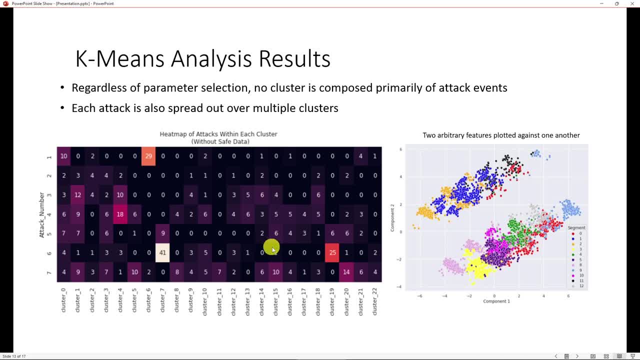 And it just skews the heat map too much, So you'll be able to see that. Also, just two arbitrary features, and I didn't label the features, so I don't know exactly which ones these are. just to see that when you kind of 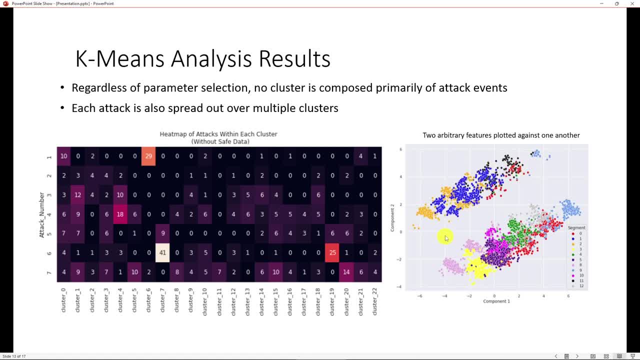 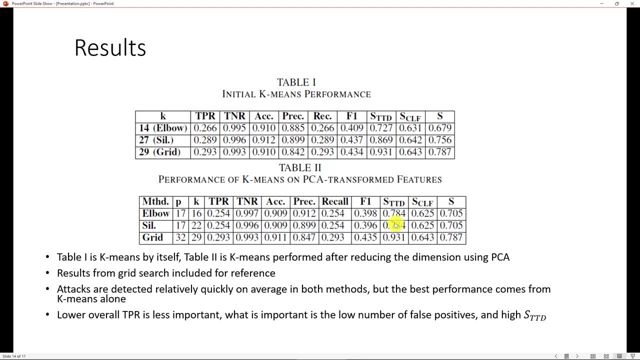 look at these things in two dimensions, it's not really clear to see where these patterns are coming from. So the results in the first one is the k-means by itself, with k selected using the ELBO method or the, what do we call it? 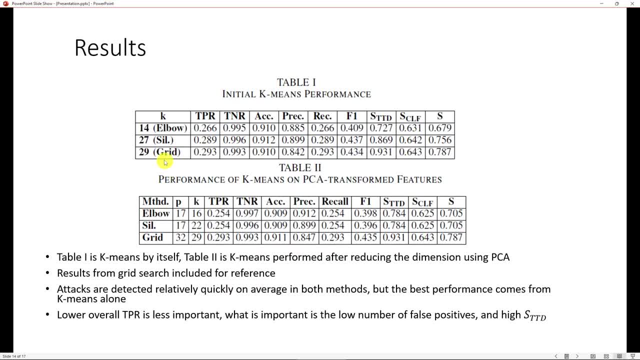 Not the silhouette score, the distortion score, excuse me, So using the ELBO or distortion scores, and then we have 27,. k equals 27 found with the silhouette score. And then we finally have the grid search, where we just looked at all the possibilities. 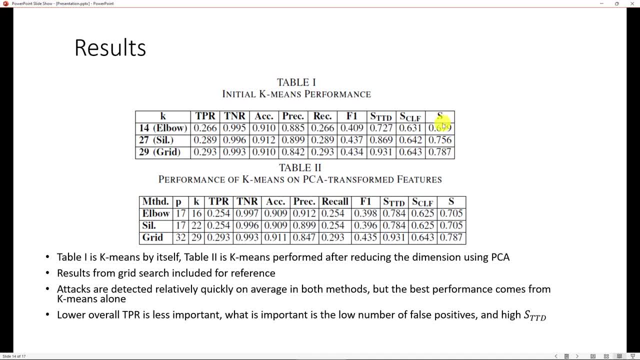 and kind of worked backwards from what gave us the highest s value. So you see, our highest one that we found without any kind of a priori knowledge is 75%, and with the best case scenario it was 78% or 79%, So not a huge distinction there. 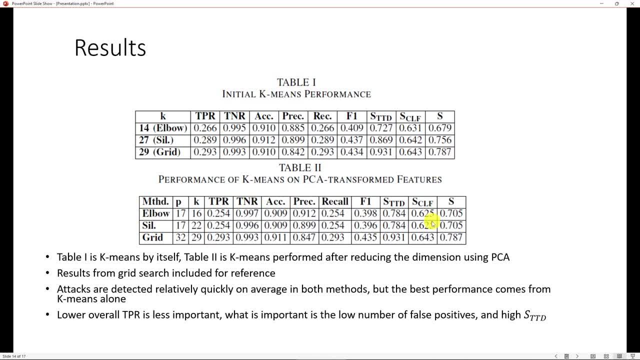 When we add in PCA, this actually lowered the performance. Let's see There's some advantage here. Yeah, So, regardless of what method. So the nice thing about this is it was less important which method we chose for selecting our parameters. They both gave the same results. 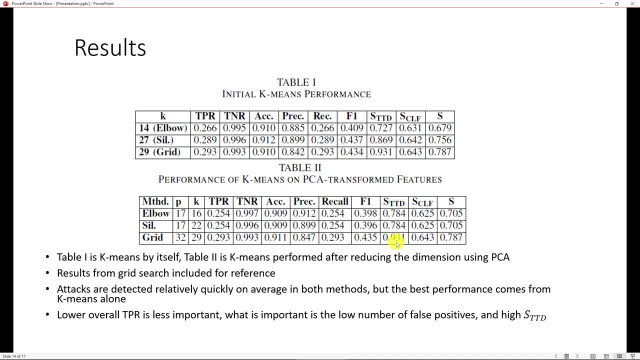 Of course, the grid search gave us significantly better results because again we're looking at the attack labels to determine our parameters. So, looking at the STTD score, or the time to detection, on average, again the k-means by itself performed very well. 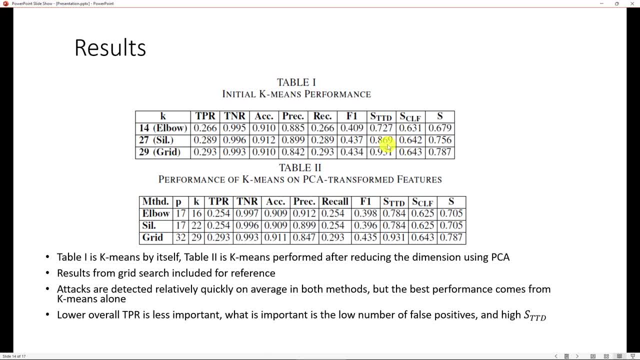 We have a score of 86.9 or So this means the attack was found in the first- roughly 13%. So very nice score. We were detecting these pretty early on. A little bit lower for PCA plus k-means at 78.. 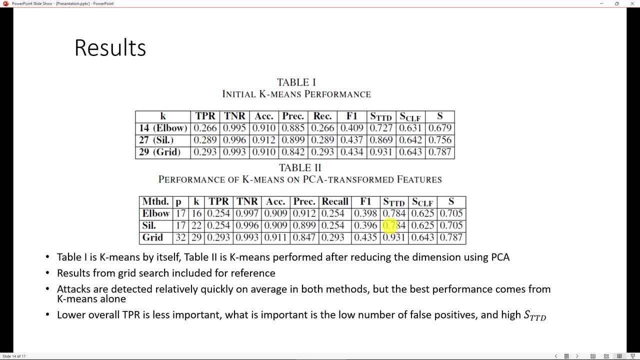 So we're detecting these attacks within the first. What is that? 21%, Again, much higher with the grid. search Other stuff. looking at normal machine learning methods- precision recall, F1, et cetera- these don't have the greatest performance. 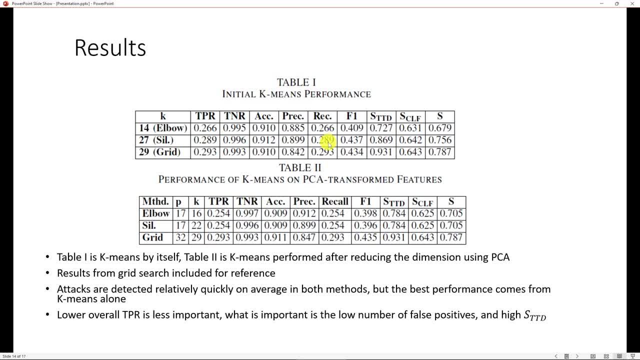 And that's because we have We're not detecting all of the attack events. You know we're getting like a smattering of these within the attack, So that leads to lower results here. But again, that's less important here, As long as we're detecting these attacks early on. 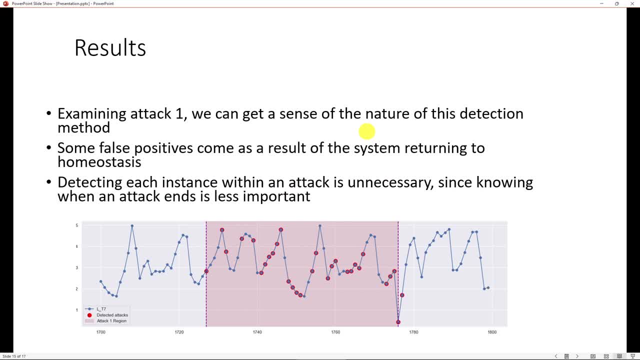 it doesn't matter if we're detecting all of the attack events. And so, looking at an example of this, we have attack one. I've got highlighted. this kind of pink window is where the attack region started and stopped, And you see that we've got pretty good. 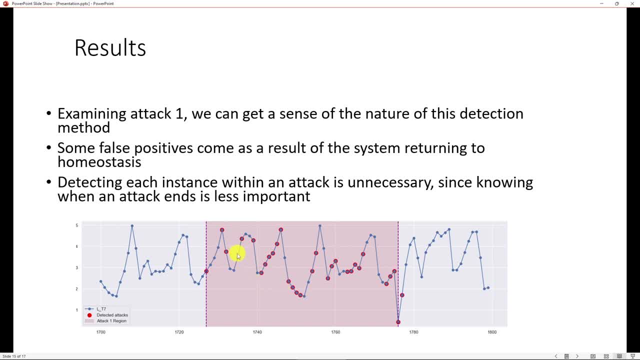 spread of attacks detected in here, And so while we're not detecting every one of these events, it doesn't matter As long as this is enough to get an operator's attention on it, to see that something is going on. then they could see, well, what's going. 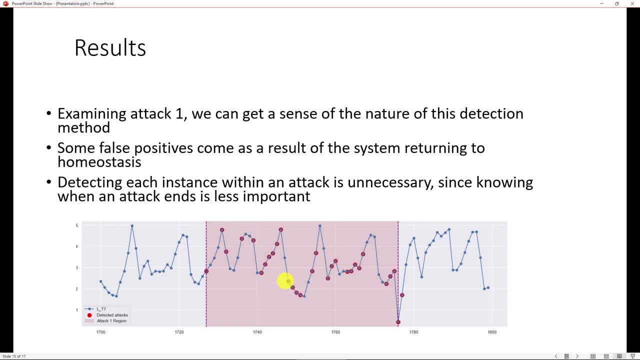 You know what is happening to our system right now. Why are we getting all these flags? And you see, these are also clustered together in pretty large and pretty nice groups here. You know, we're getting a string of flags, all one after the other. 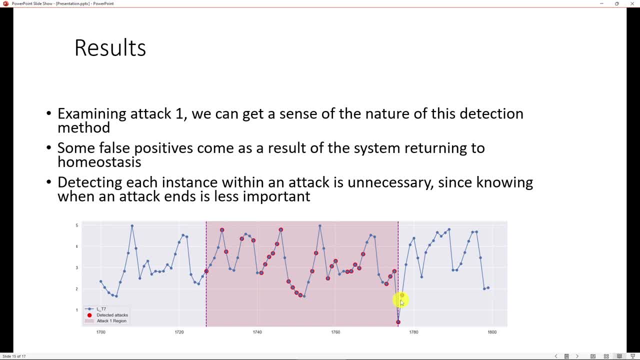 Other things to note here, and this is common: after an attack ends, it takes some time for the system to return to like homeostasis or normal operation, And so we do get some false positives here that aren't really false positives. 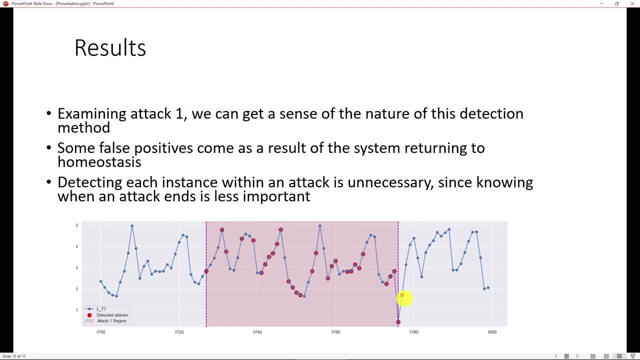 because things are still performing unusually, even though the cyber attack itself has ended. This is a nice thing to note as well. So some of these false positives are actually lower, And we had very few false positives using this method. Yeah, so looking at this again, 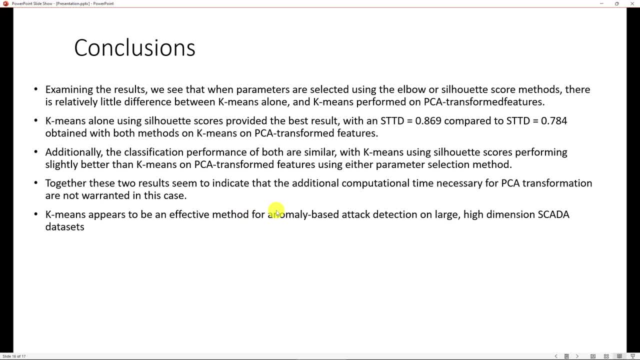 I've essentially gone over these things. There's relatively little difference between k-means alone and k-means performed on PCA-transformed features. It doesn't seem to be necessary to do this. It performed just as well and in fact better. 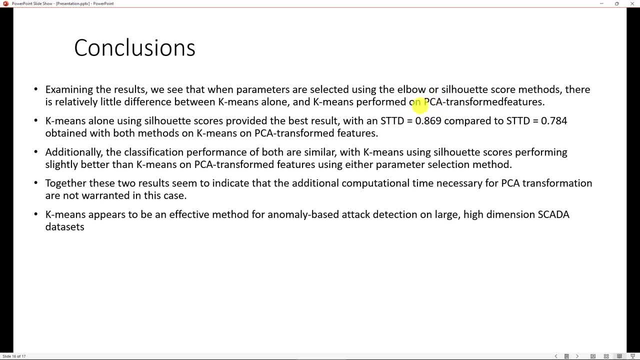 without adding in this addition. So this is just an additional step. Using silhouette scores provided slightly better results: 0.869 times detection over 0.784. And that had a pretty large effect on the overall score, Although the classification was very, very similar here. 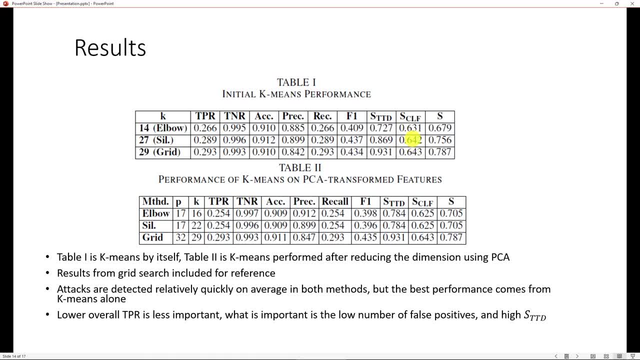 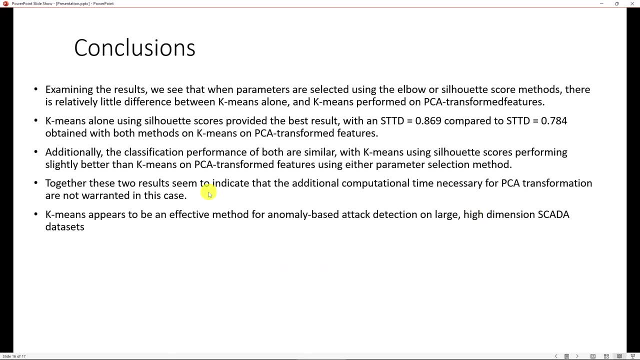 Right, our classification score 0.64.. In the best case here And 0.625,. best case here: Yeah, so I already said this, The additional computational time necessary for PCA transformation is not necessarily warranted. But yeah, altogether, this method was reliable. 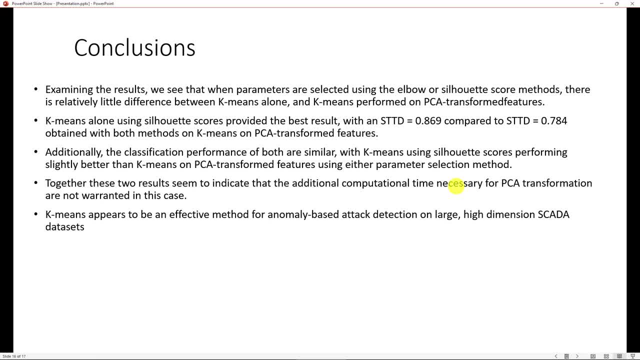 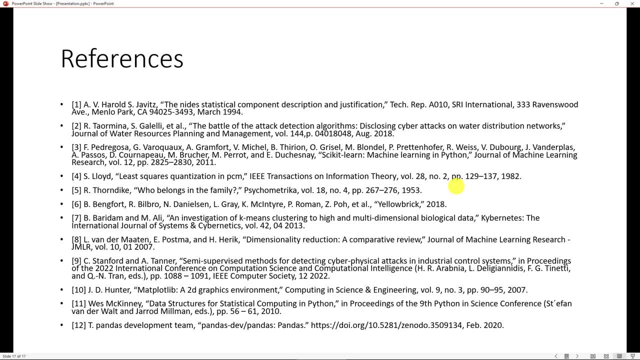 It detected each of the attacks. We didn't miss any here, Although it may have missed events within a particular attack. Just a list of references here, And that is it. Thank you for your time.